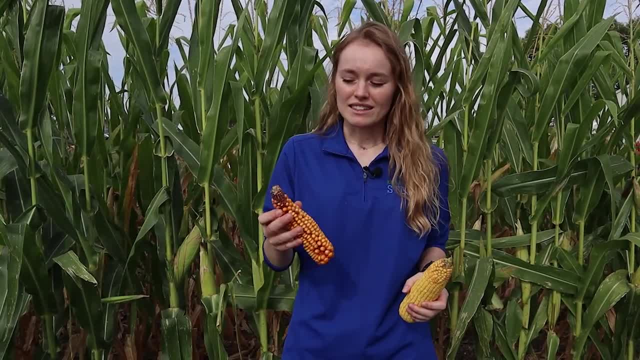 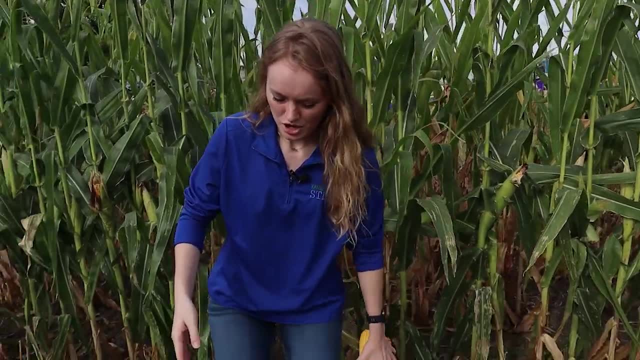 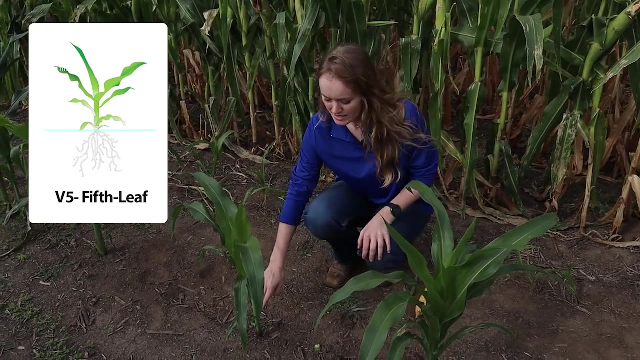 talk about in a minute, but they wouldn't be pollinating at the same time, which means you may not have enough pollen to fill those ears When we get to V5, like this plant here. this is important because during this time the stem in corn first comes above the ground, which is kind. 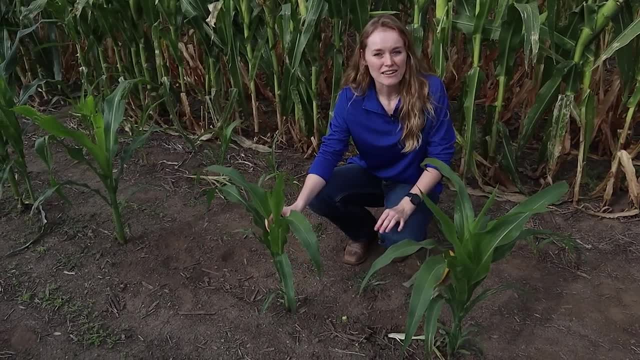 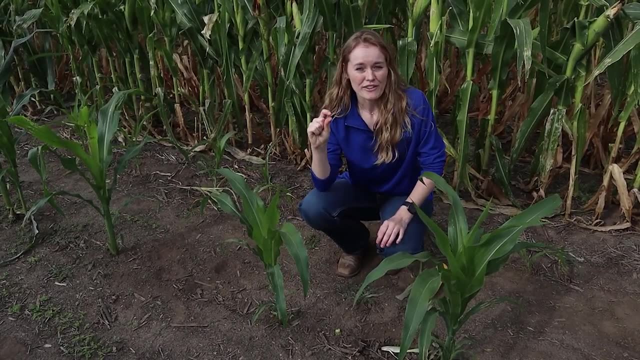 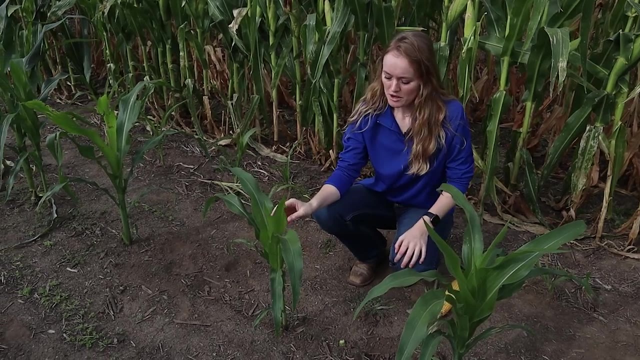 of strange to think about, But this plant as a V5 plant. everything you see here is all leaves. The stem is very, very small. At V5 is when that stem starts to have its growth spurt and the stem actually starts growing above the ground. This is important because once that stem comes above, 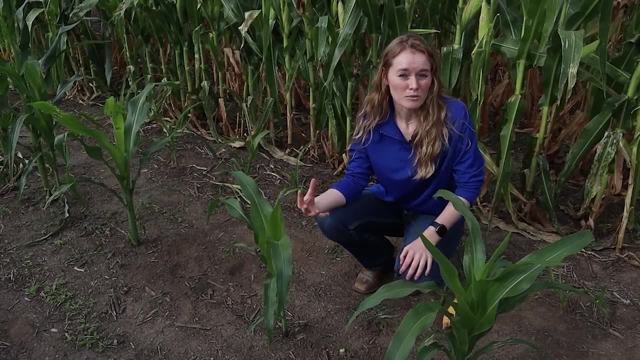 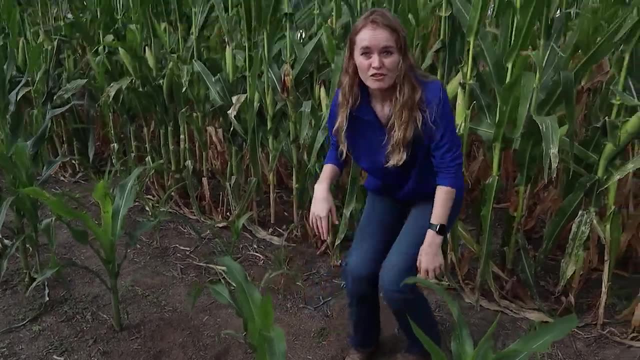 the ground. anything that damages this plant can start to grow above the ground. So if you're looking at a plant that's growing above the ground, you can see that it can do permanent damage to that plant when we start looking at ear development. So that's really, really important. 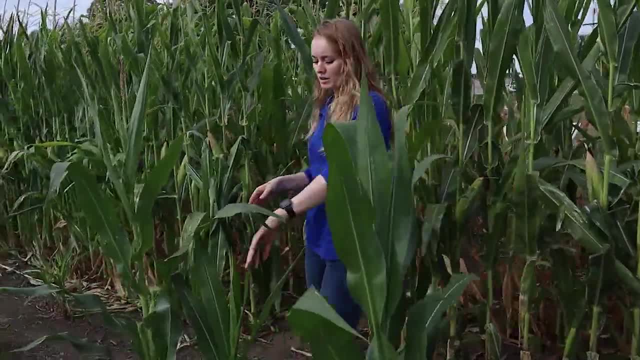 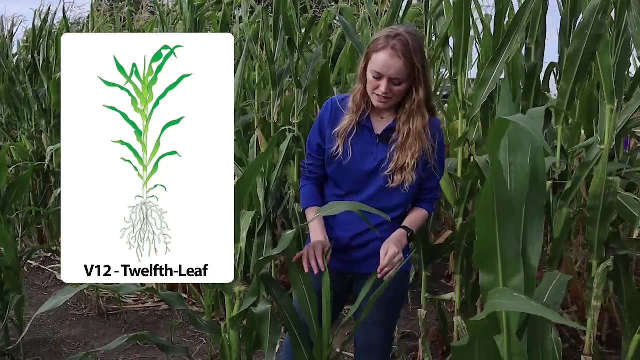 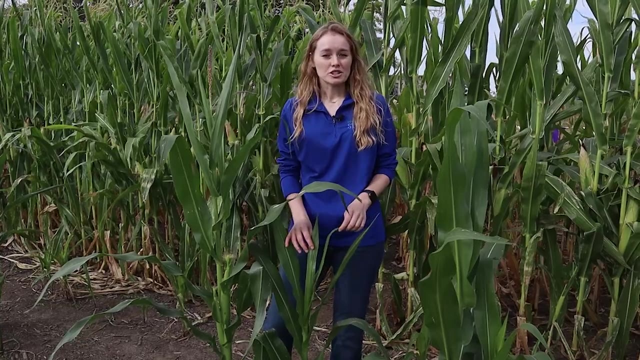 If we come over here, we can see some other stages of corn that we're going to be looking at. This plant is V12, which, if you'll recall, means it has 12 collared leaves. At this point, the ears are really starting to develop inside of this plant. We can't see them yet, but it's already. 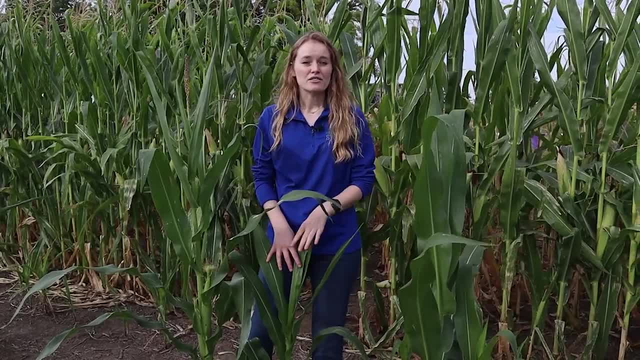 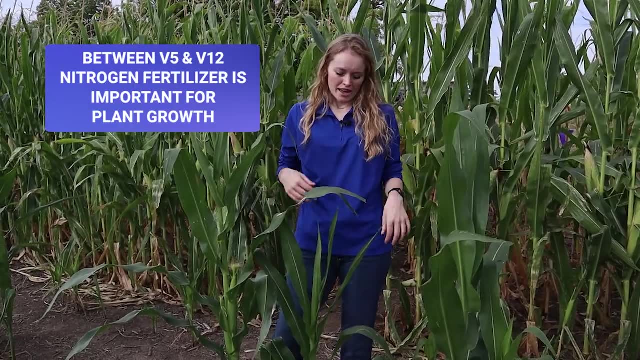 determining how many kernels are going to be on each of those ears Between V5 and V12, nitrogen fertilizer is something that's really important. The plant starts growing a lot and these green leaves. there's a lot of nitrogen that's in these leaves. 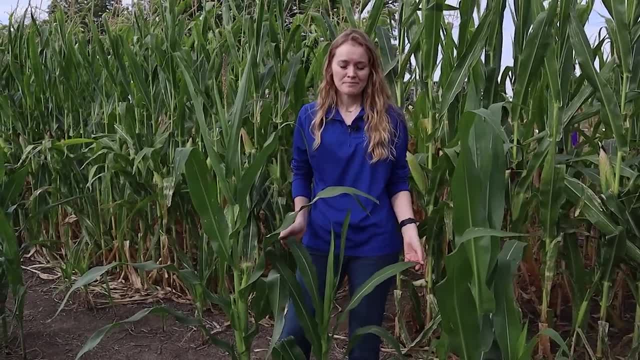 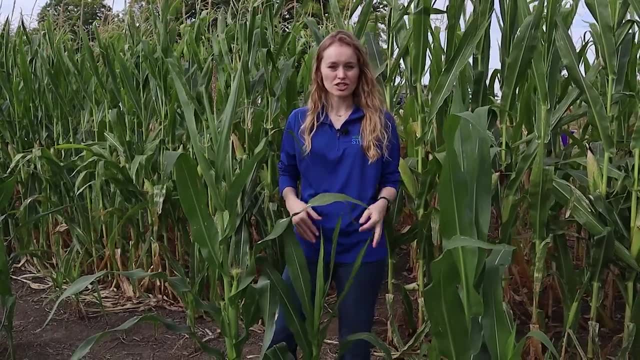 which means fertilizer is really important during this time. After plants get to be about this, big weeds aren't as much of a concern because the leaves start taking up more of the light, which means less of it can reach the ground and weeds aren't. as important. So if you're looking at a plant that's growing above the ground, you can see that it's growing above the ground, which means less of it can reach the ground and weeds aren't as important, doesn't get as competitive at that point. 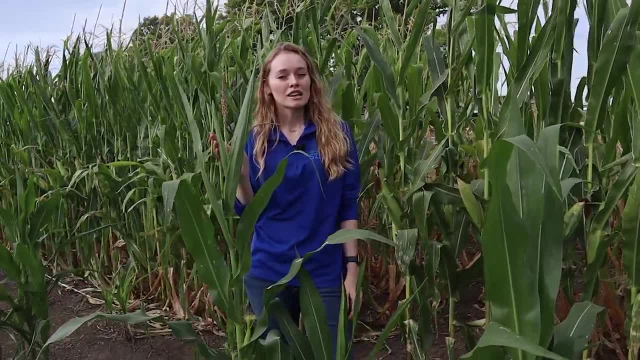 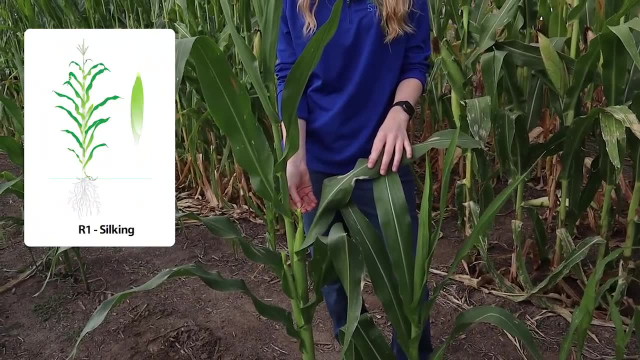 This plant will continue growing until we see a tassel popping out the top and silks coming out of our ears. When we see silks coming out of our ears, we know that we've reached R1, reproductive 1, the first stage of the reproductive cycle. But you also need to understand that we're 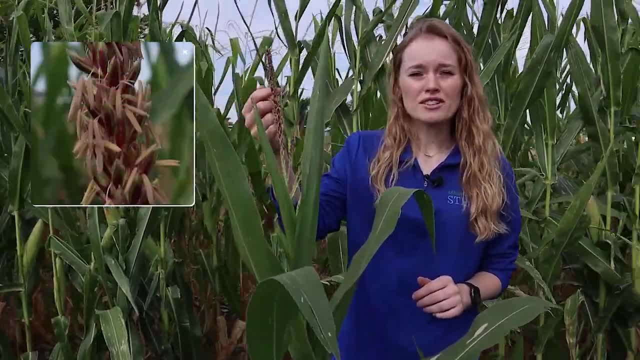 ного of an air. Don't let it ruin your 7 honey. But you also need to understand that we're even more likely to have colonies of a different variety of ermigones villainizing the whole soil. We can see on this tassel: we have some anthers that have popped out of this corn tassel.